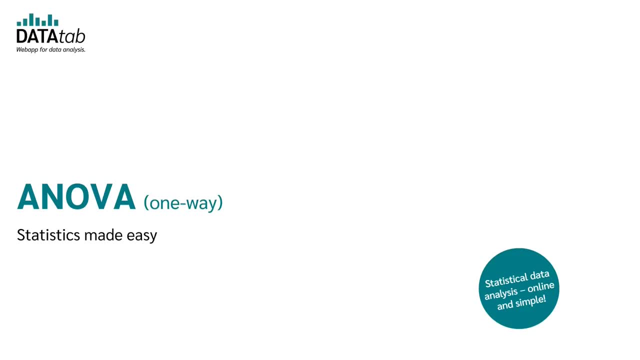 Hello, in this video, I explain to you in a simple way what an ANOVA is and how you can calculate it. To be precise, it is about the simplest form of the ANOVA, the one-way ANOVA, and that's where we start. 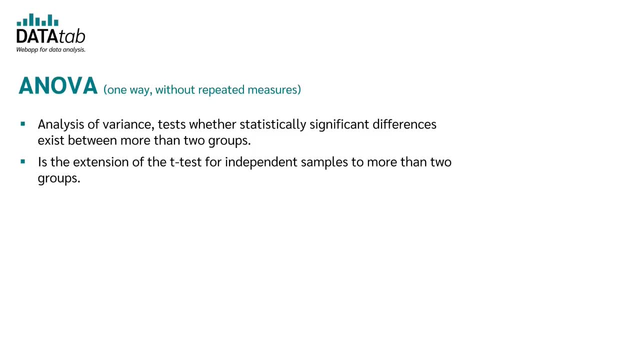 First, why do we need an ANOVA at all, Or what does an ANOVA do? Analysis of variance checks whether there is a statistically significant difference between more than two groups. Thus, analysis of variance is the extension of the t-test for independent samples to more than two. 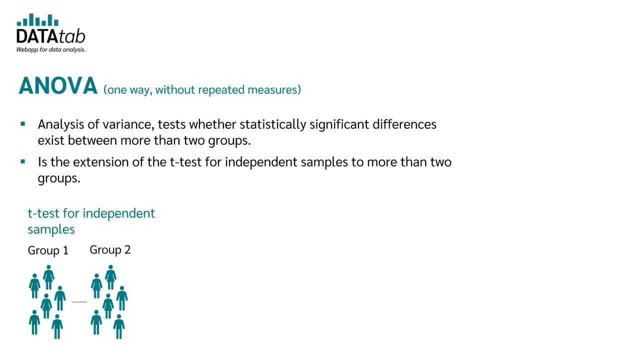 groups. In the independent t-test, we looked at whether there is a difference or, more precisely, a difference in means between two groups. For example, there's a difference in salary between men and women. In this case, we have two groups: the men's group and the women's group, If we want. 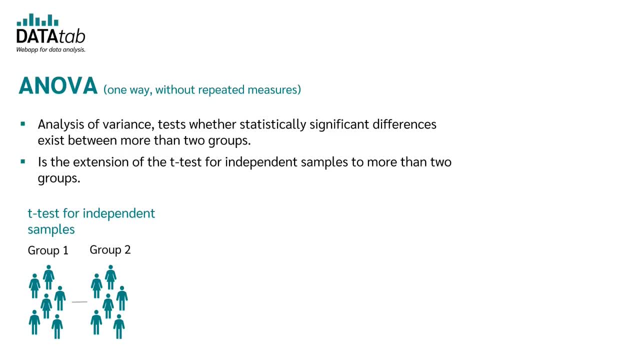 to compare more than two groups. we need to compare the difference between two groups, So we use the analysis of variance. The addition in the t-test for independent samples is the same as the addition in the analysis of variance without repeated measurements In the t-test. 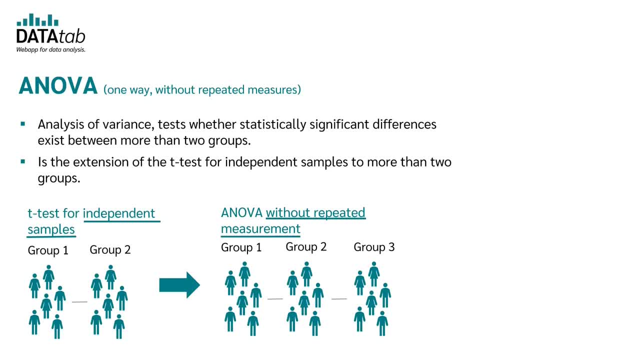 we used an independent t-test if the two groups or samples are completely independent, For example, if one person in this group has nothing to do with the person in this group. Exactly the same now applies, the analysis of variance, without repeated measures, except that here we have at least 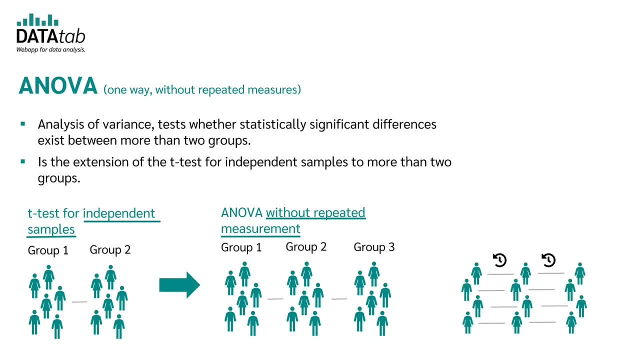 three independent samples. We would have dependent samples, for example, if the same person in a group were interviewed at several points in time, Then we would use an analysis of variance with repeated measures. But now let's look at a few examples. A classic application for analysis of variance is in therapy research. 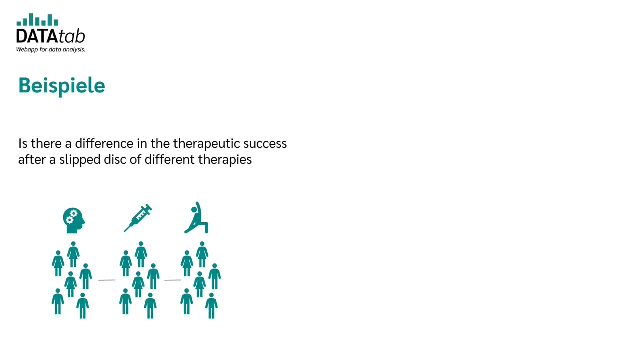 For example, you might be interested in whether different therapies result in different therapeutic successes. The question could be: is there a difference in the therapeutic success after a slipped disc of different therapies? On the one hand, you can discuss with patients which movements are good and which movements 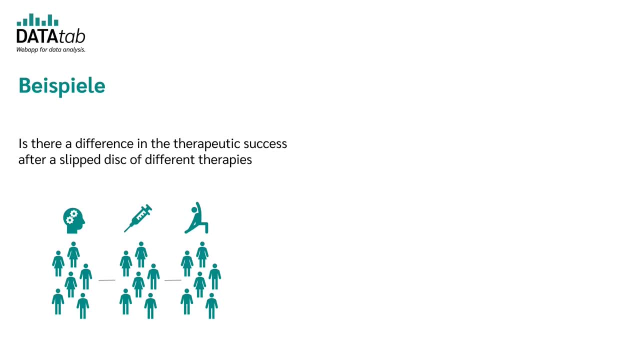 are bad for a slipped disc, Then you can treat one group with medication and with the last group you can do stretching and strength training. At the end of the therapy, you could then investigate the success and calculate, with the help of the ANOVA, whether there is a significant difference between the three forms of therapy. 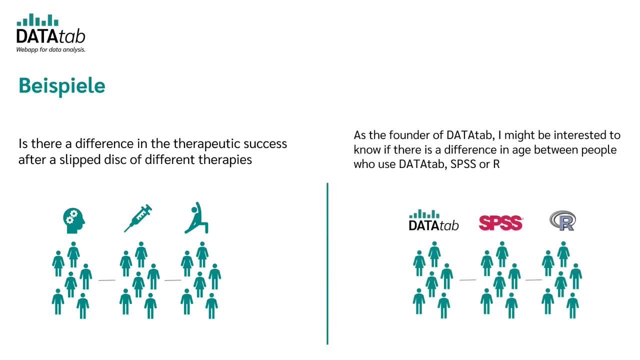 And now an example from marketing. As the founder of DataTab, I might be interested in whether there is a difference in age between people who are using DataTab, SPSS or R. For this I take a random sample of people who use statistical software. 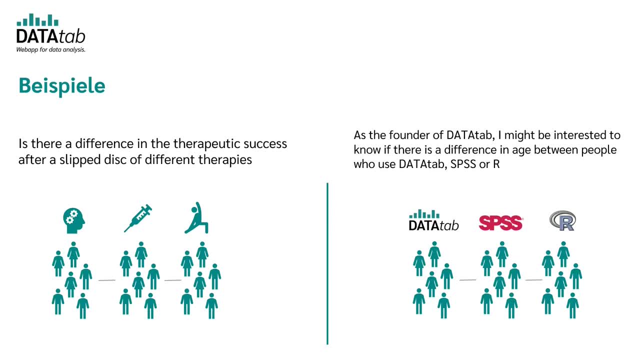 Then I ask them which statistical software they are using and how old they are. So I have the group of people who use DataTab as a statistical software- SPSS and R- And I want to know if there is a difference in age among these groups. 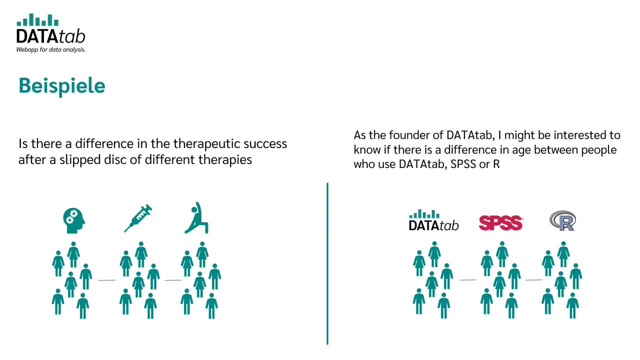 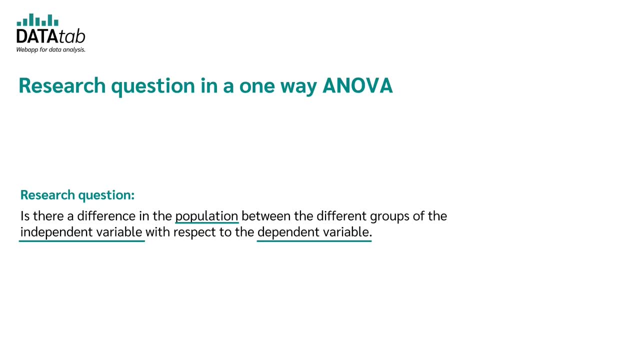 I have only taken three groups, but of course you could use also more groups. What exactly is the research question in an ANOVA? The question is: Is there a difference in the population between the different groups of the independent variable in relation to the dependent variable? 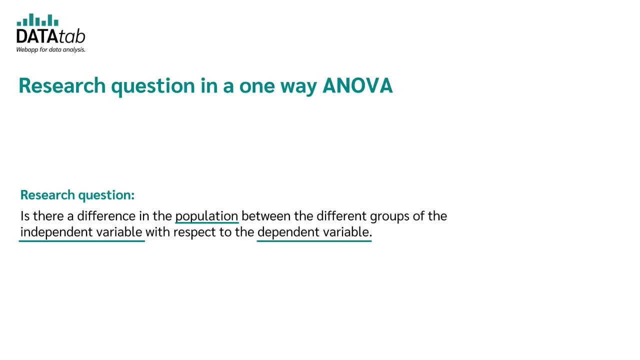 Don't worry, we will go through the sentence briefly. You are probably wondering why population, what is the independent variable and what is the dependent variable? The independent variable is the variable with the different categories, So in our example it is the therapy type. 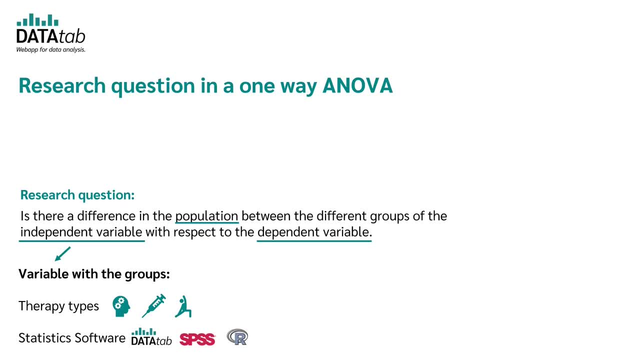 With the group which learned the right behavior For a slipped disc, the therapy with medication and the strength therapy. In the second example, the independent variable is the statistical software used with the groups DataTab, SPSS and R. The dependent variable in our example was: 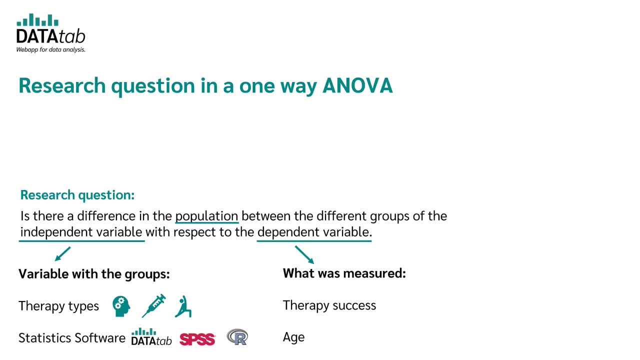 the success of the therapy and the age. We would like to know whether the groups of the independent variables have an influence on the dependent variable. Therefore, For our two examples, the questions would be: Is there a difference between the different types of therapies in terms of the therapy? 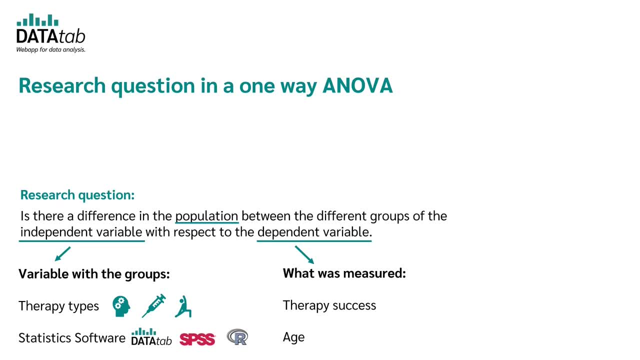 success, Or Is there a difference between the users of different statistical software solutions in terms of age? Now the last point: why population? Actually, we want to make a statement about the whole population. Unfortunately, in most cases, it is not possible to survey the whole population. 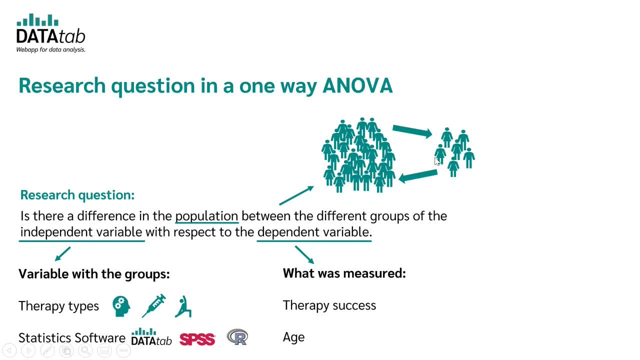 And we can only draw a random sample. The aim is to make a statement about the population based on the sample with the help of an ANOVA. Of course, we did not carry out the experiment on therapy success with all people who have a slipped disc, but only with a random sample. 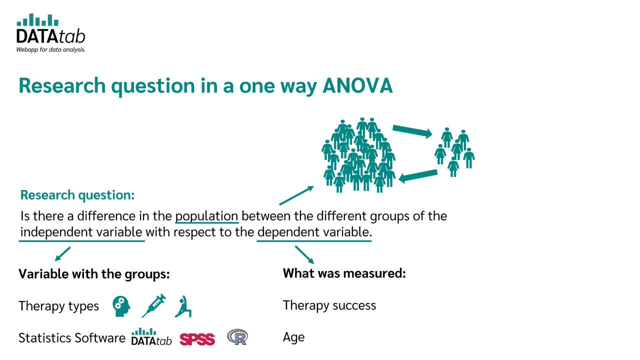 But we would like to generalize the statement for the population. Therefore, we use the ANOVA and check whether the result is significant or not, And we can only draw a random sample. The aim is to make a statement about the population based on the sample. 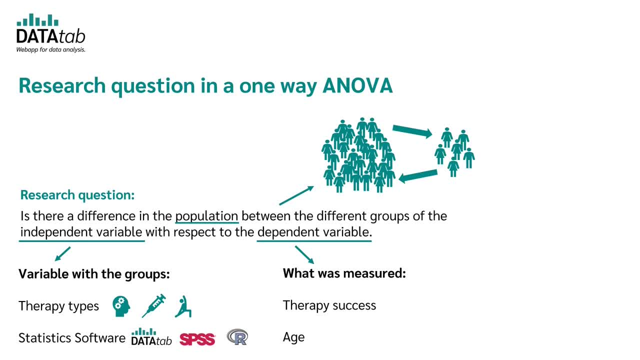 And we can only draw a random sample. Therefore, we use the ANOVA and check whether the result is significant or not, And we can only draw a random sample. Therefore, we use the ANOVA and check whether the result is significant or not. 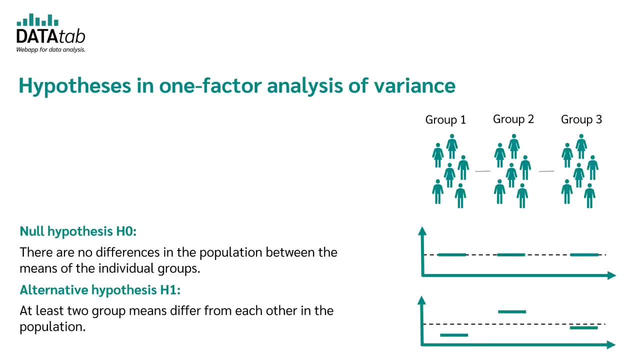 Now we have understood this, we move to the hypotheses. Before you calculate an ANOVA, of course you have to make the hypotheses. In the case of the analysis of variance, the null hypothesis is that there is no difference between the means of the individual groups. 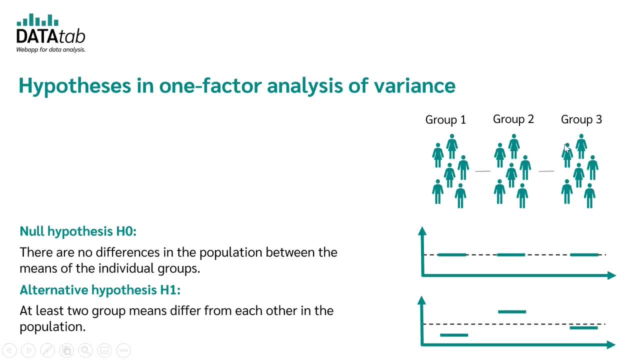 We have our groups, of which we can calculate the mean in each case, And our null hypothesis is now that there is no difference in the means of the individual groups. The alternative hypothesis is that there is a difference between the group means, In other words, there is a difference in the mean between the groups. 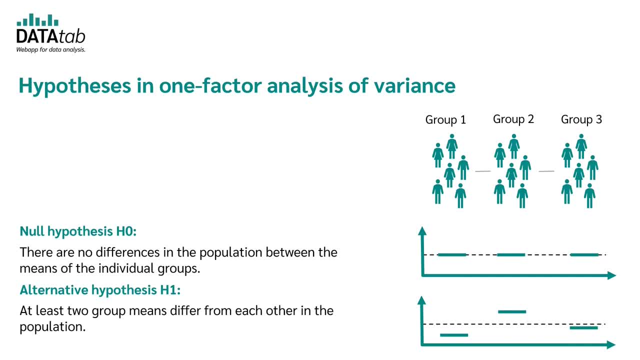 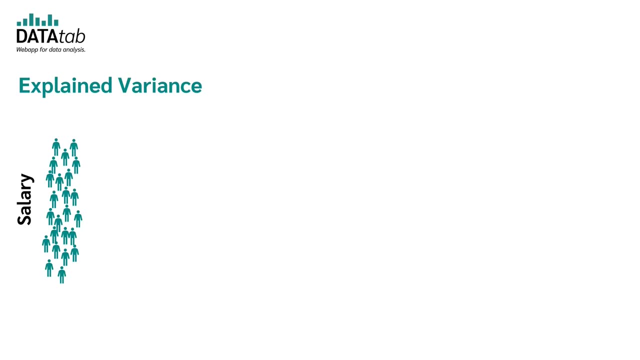 Therefore, our null hypothesis says that there is no difference and the alternative hypothesis says that there is a difference. All well and good, now we know what the null hypotheses are, But what does it mean exactly? Let's say, we want to test whether there is a difference in the salary between these three. 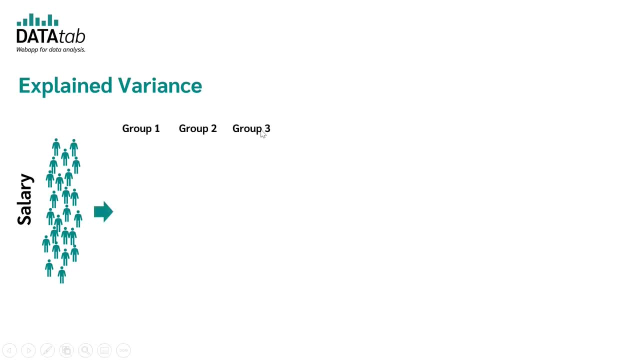 groups: Group 1,, group 2 and group 3.. Now, of course, the salary has some variance. Some people earn 500 euros a month, others earn 2600 euros a month, or some people earn 6000 euros a month. 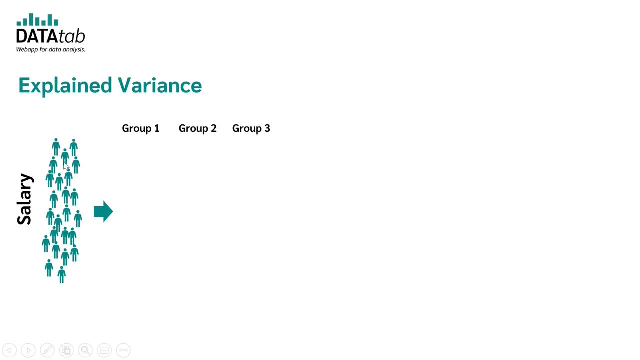 So both in the population and in our sample there is a variance in the salary. Now the question is: where does the variance come from And can we explain some of these variations by the three groups? So how much of the variation in the salary can we explain by dividing the people into 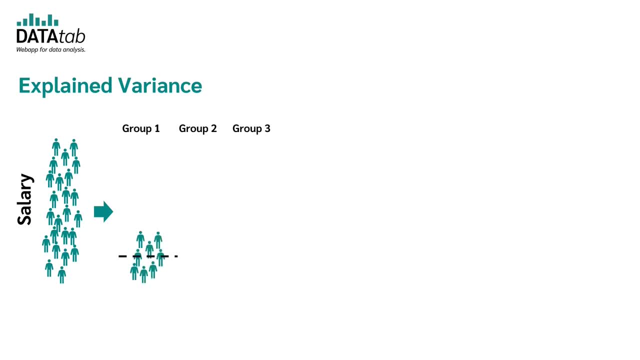 these three groups. In the extreme case, the results could be that the salary in group 1 is distributed like this, in the second group like this and in the third group like this. In this case, the division into the groups could explain a lot of variations. 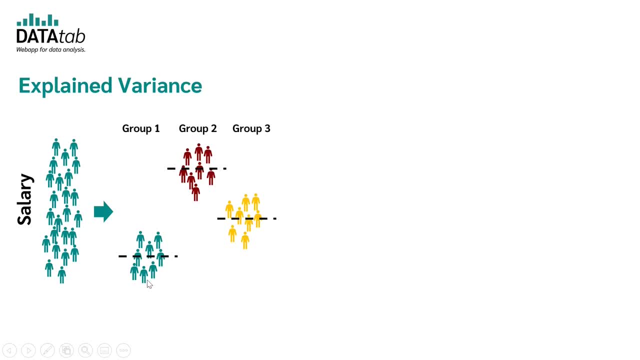 For example, let's say we have a small variation in the salary. We have only a small variation in each group. The result would be different in this case. Here we would again have the variable salary and would divide it among three groups. Here, however, we could explain almost no variance by forming the three groups. 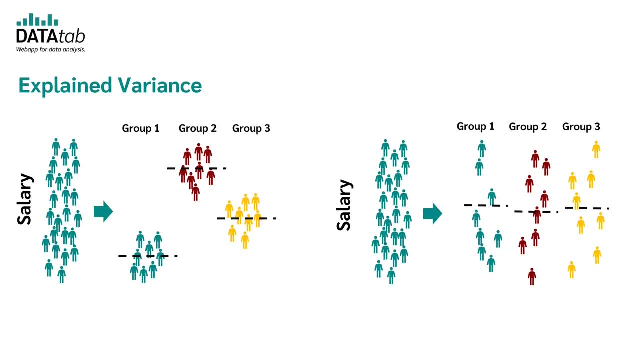 Within the groups the variance is almost as the same as in the whole sample. So it does not matter whether we form the groups or not. We can extend it further to make sure we have the test the same way as before. If we look at the variance between the groups, we can establish that in this case there is 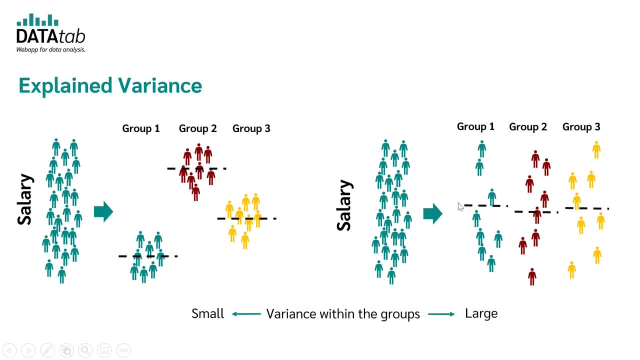 a big variance, And in this case there is a big variance in the people in the first, and so the variance is also large. Wir sehen, wie wir den Chuck primeira Seunglistung auf spohlichen Gelände aus después des Versuch olduğmer Um. 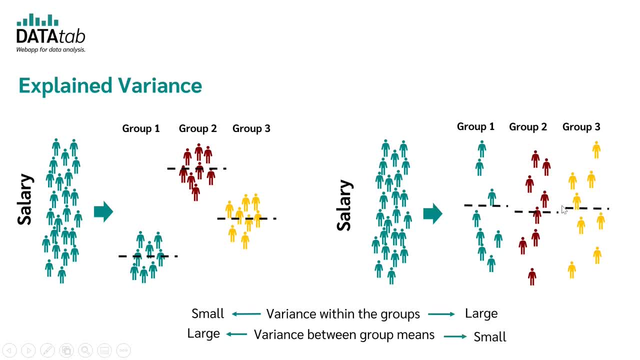 erfahren können, Angesóbig in this case. Here, the means of the groups are not far away. Now, of course, you want to know how you can calculate an analysis of variance. There are two possibilities for the calculation. Either you can use statistical software like 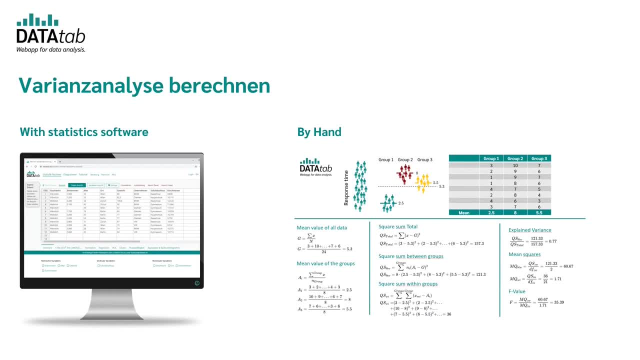 DataTab or you calculate the analysis of variance by hand. To be honest, no one will calculate the analysis of variance by hand, but the knowledge is very useful to understand more precisely how an analysis of variance works. In this video, I show you how you can easily calculate an analysis of variance online with 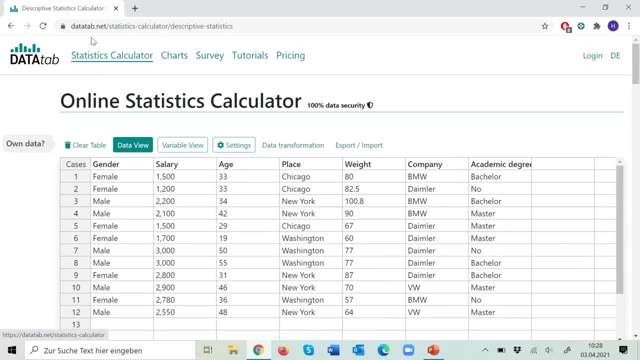 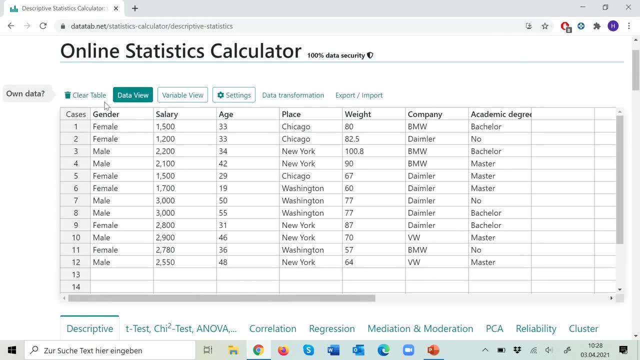 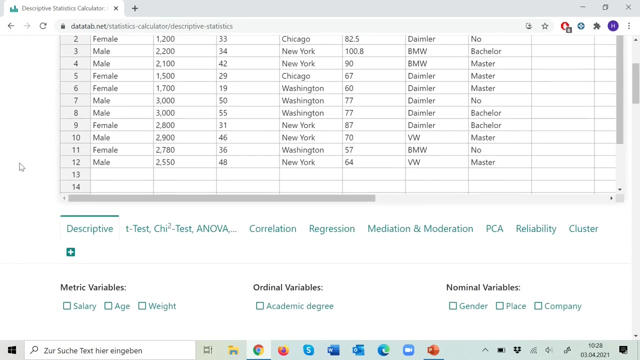 DataTab. To do this, just open data tab dotnet and click on the statistics calculator. If you want to use your own data, you simply need to clear the table and put your data into this table. I will use the example data because we want to